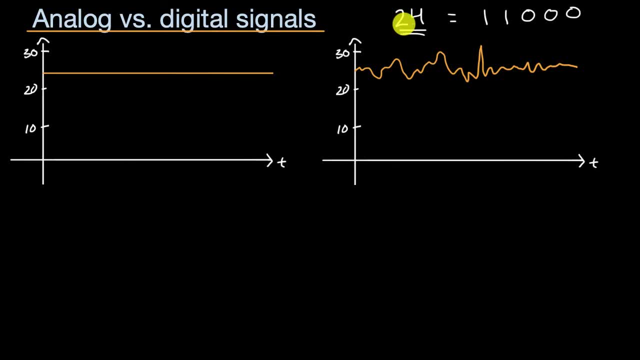 that explain how to convert back and forth between our decimal system that has 10 digits, zero through nine, and the binary system, which has two digits, zero and one. But in case you're curious and you don't have to understand this, 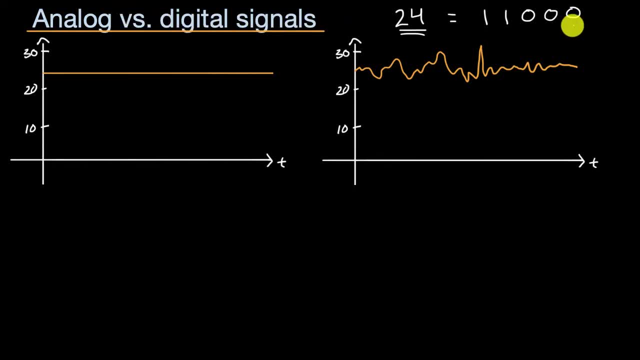 to know the difference between analog and digital signals and when they might be useful. this first place is the ones place, just as you're used to, But instead of this being the tens place, this is the twos place, Instead of this being the hundreds place. 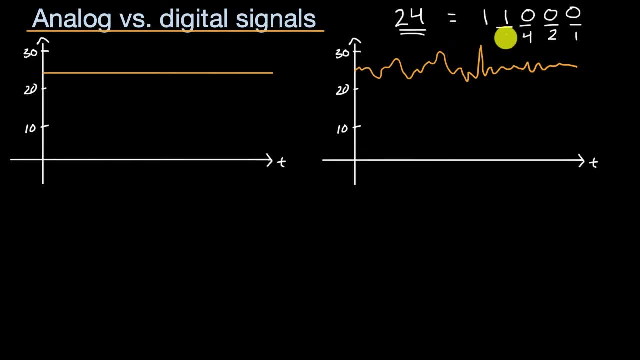 this is the fours place. Instead of this being the thousands place, this is the eights place, And instead of that being the ten thousands place, that's the sixteens place. So one way to think about it: 1 1 0 0 0 means 1- 16 and 1- 8.. 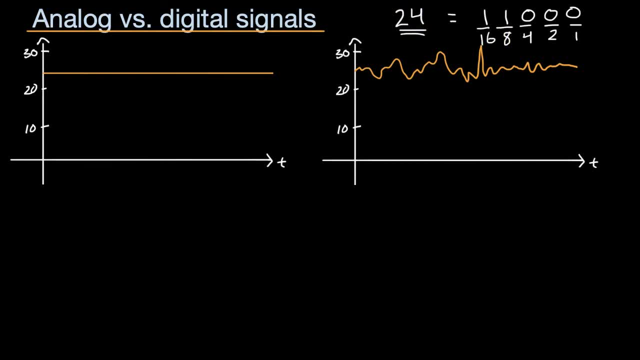 And if you add those together, you would get 24.. What would that actually look like as a signal? Well, it could look something like this, where the person interpreting it knows that over this first time period, whatever voltage you're getting, 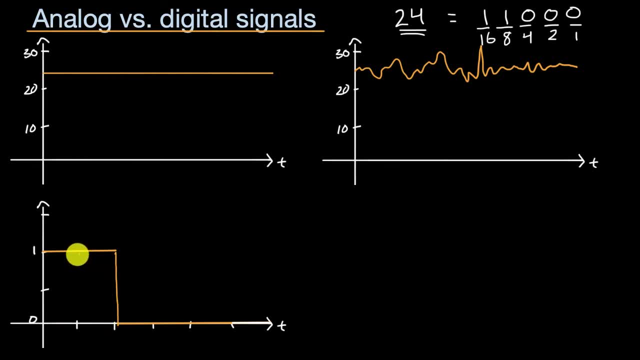 that tells you your first digit, Then over the next time period, whatever voltage you're getting, tells you the second digit, and so on and so forth. So this would be 1 1, 0, 0, 0.. Now why is this useful? 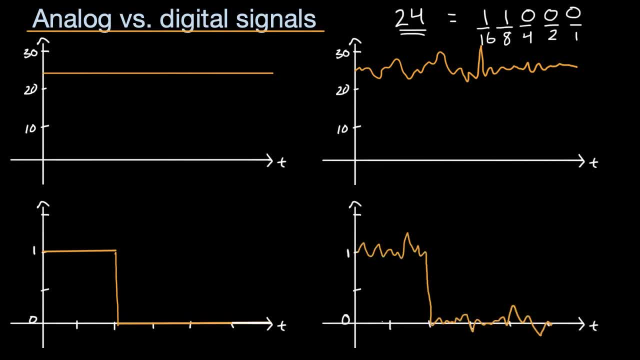 Well, let's think about the situation where, all of a sudden, there's interference again. Now, with the interference, you could still interpret this exactly as 1, 1, 0, 0, 0.. Remember the person receiving the signal or the system receiving the signal. 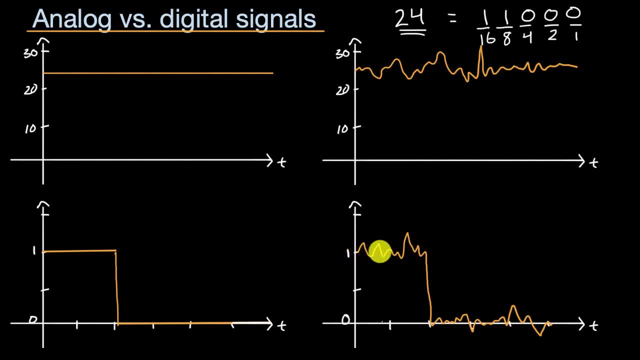 is just trying to determine whether it's getting a one or a zero. So even though this is being perturbed right over here, it's clear that we are at a one. We know that it would not be a 0.9 or a 1.1.. 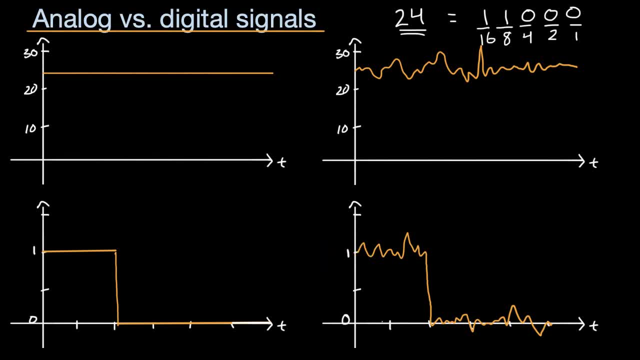 It has to be either a one or a zero. So it's clear that over this part, right over here, you're getting a one, and then over here you're getting a two, You're getting three zeros. So they would be able to interpret it as 1: 1, 0, 0, 0,.